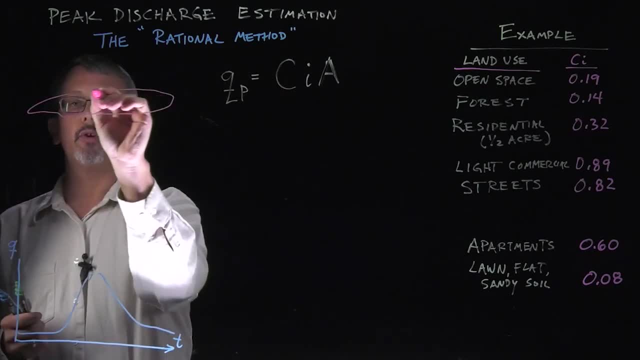 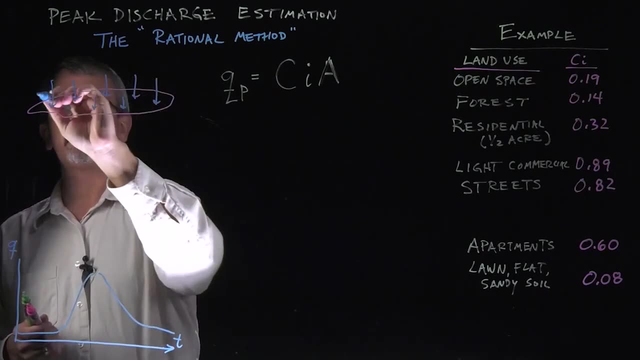 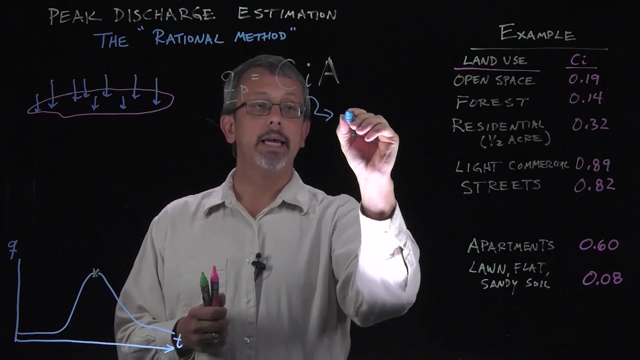 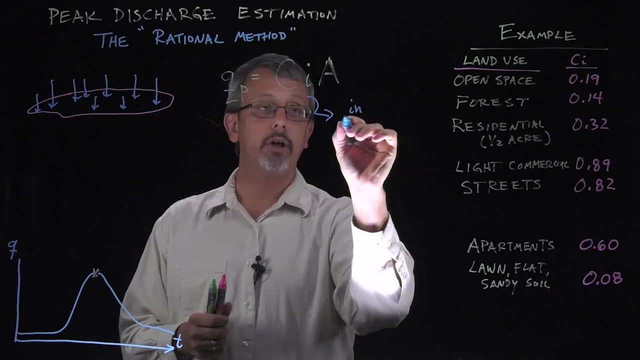 that area is if we're thinking about the rainfall falling on some two-dimensional area with a particular intensity. and now the intensity we're talking about is a measurement we've seen a little bit before, which is usually a measurement in of inches per hour. it's some measurement of depth of rainfall fall in some units. 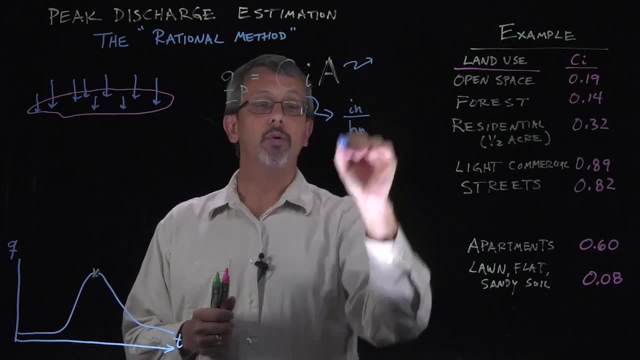 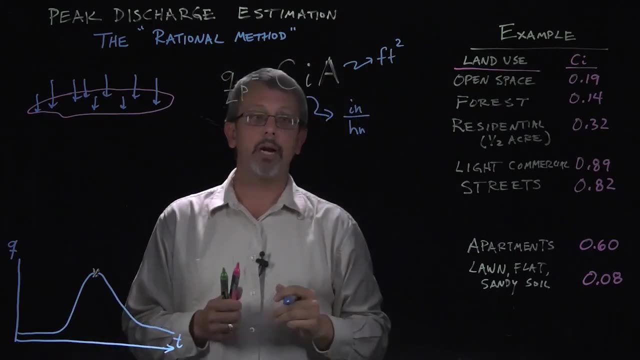 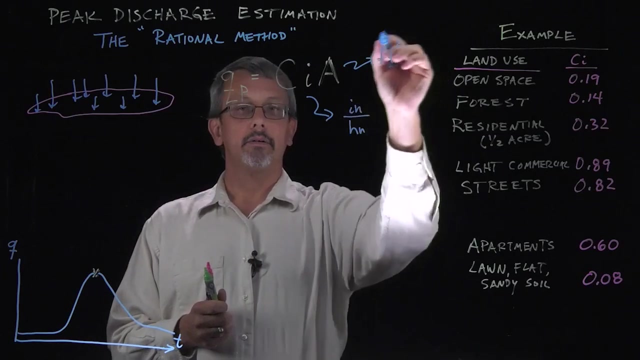 of time, inches per hour, and then again our area is going to be in some sort of area, maybe acres, maybe feet, it might be some square feet or something along those lines. inches per hour, square feet. okay, and notice, if we do that we're going to get a flow rate in volume: feet cubed times, inches or feet square times. 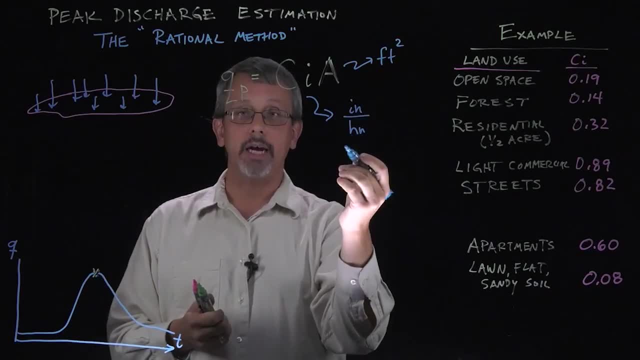 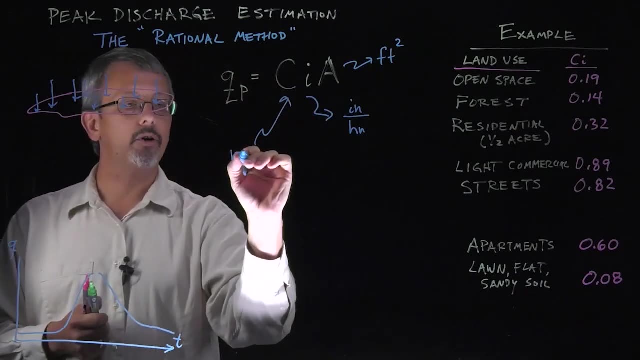 inches would be cubic feet if we do the right conversions- volume over time. so this is going to end up being something in volume over time and then we simply have this number of feet per hour and then we're going to get a flow rate in form of a Works Incorporated improvement representation. so we know how much. 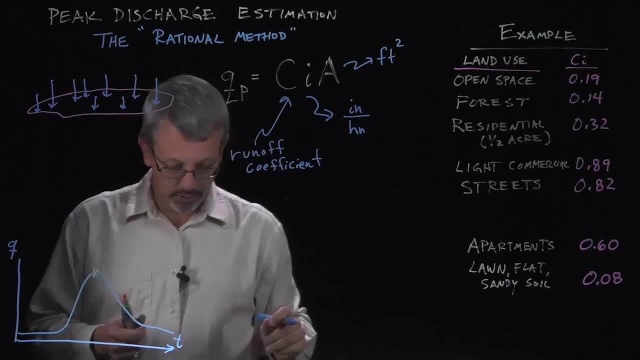 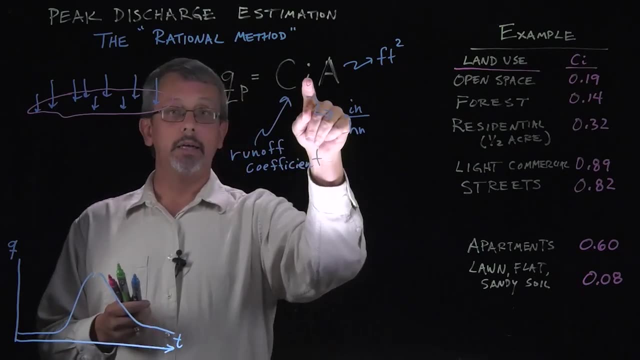 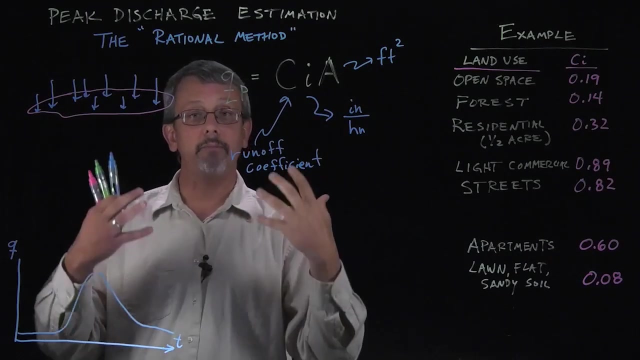 foot violate the body, works in the body. so to root that into the four part order. so if we could get a flow rate in time here, we would calculate it then and be able to do some technique to get our flow rate in alignment with the policies that we offer. and of course you never know how long it's going. 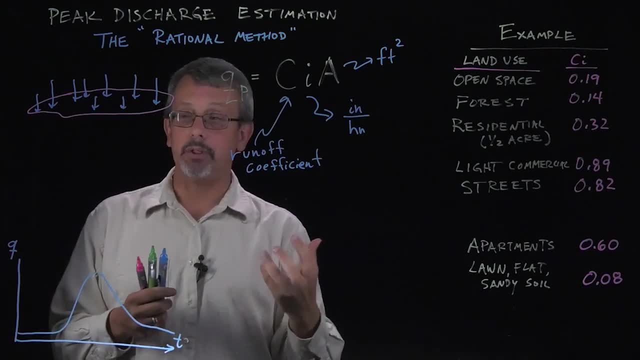 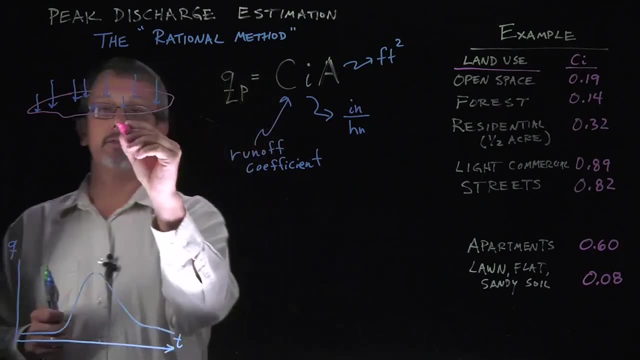 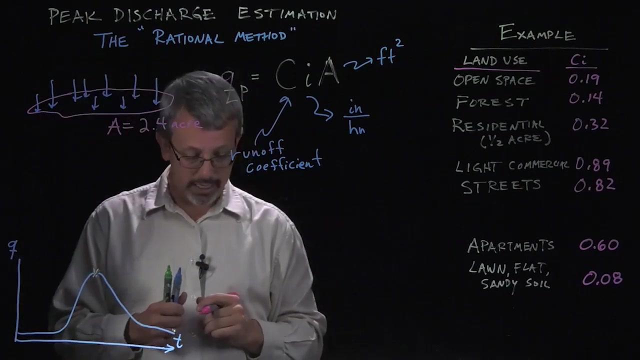 to be going to be going on, don't you know? I'm not adding to this experiment, so let's do another thing: what percentage of its going to runoff? for example, let's say we had a plot of land that has an area of 2.4 acres. we have some sort of 2.4 acre plot of land. 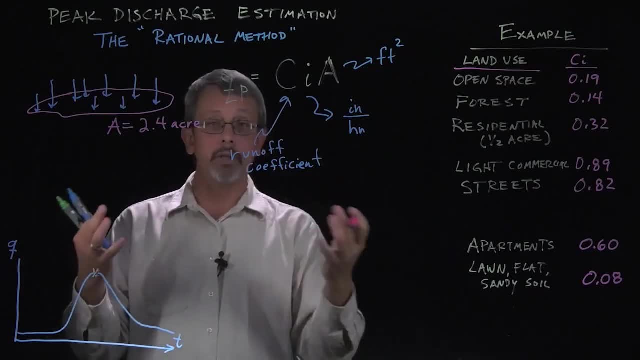 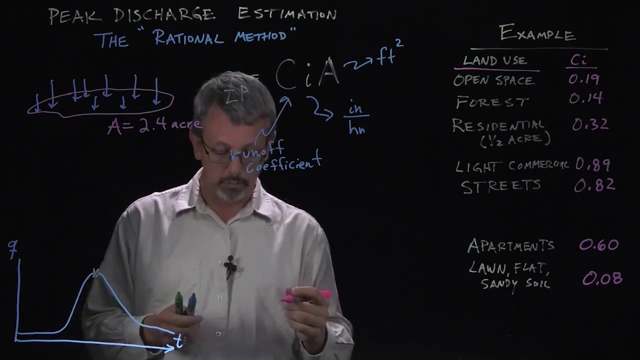 and a storm comes through. we'll call it a 25 year storm, something we assume every 25 years comes through. storm comes through and we'd like to know what our peak runoff is going to come from this 25 year storm, and we look up our 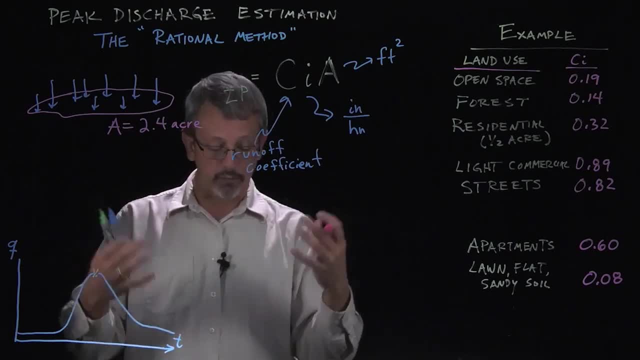 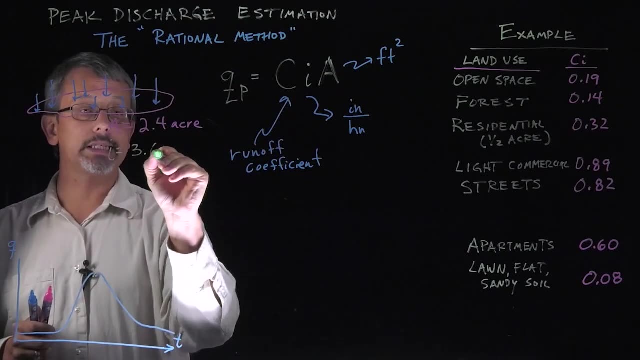 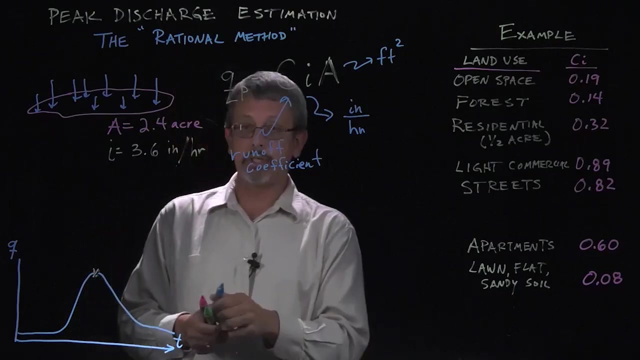 intensity, duration, frequency curves, and we find out that a 25 year storm in a particular area might have an intensity of 3.6 inches per hour. well, what I'm going to do is I'm going to consider the volume, the total volume that's going to. 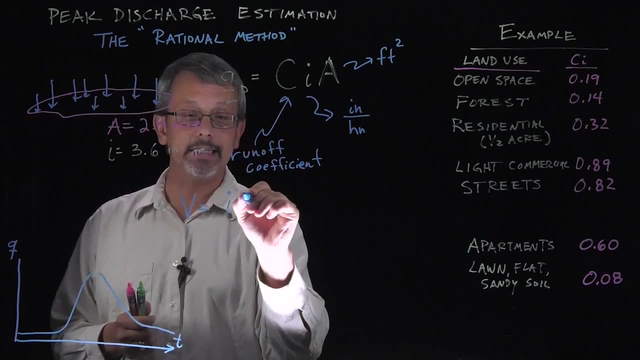 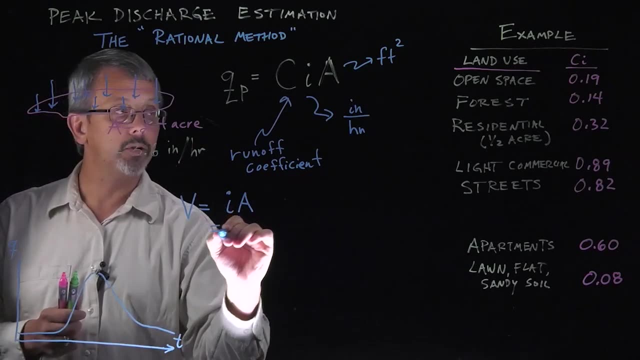 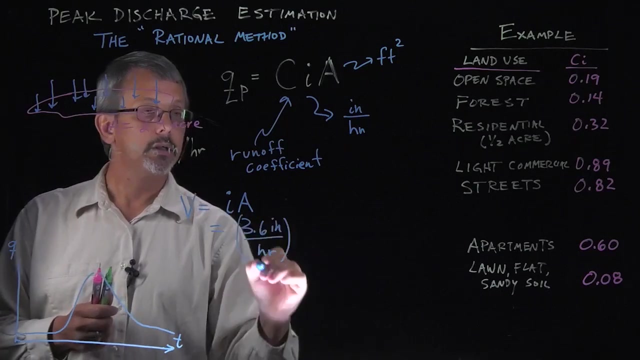 fall on this particular area is going to be equal to that intensity times the area. so V equals I, a volume equals intensity times area. so we multiply our three point six inches per hour times the area of two point four acres, and now we're going to need to do some conversions to actually get an appropriate set of units. four thousand four, I'm sorry, forty three thousand five hundred and sixty feet in an acre. okay, as well as conversions, for one foot is 12 inches and one hour being 3600 seconds. if we actually want to do this and if we do that calculation, we multiply all those numbers out. we might. 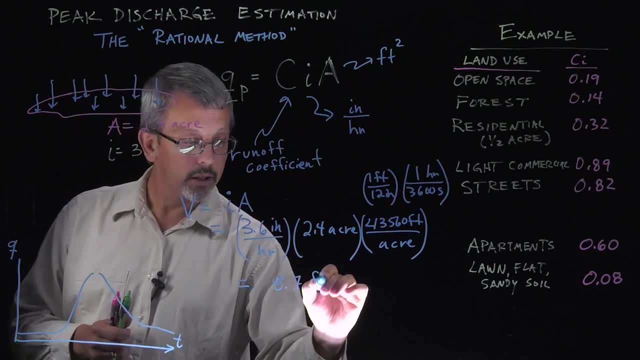 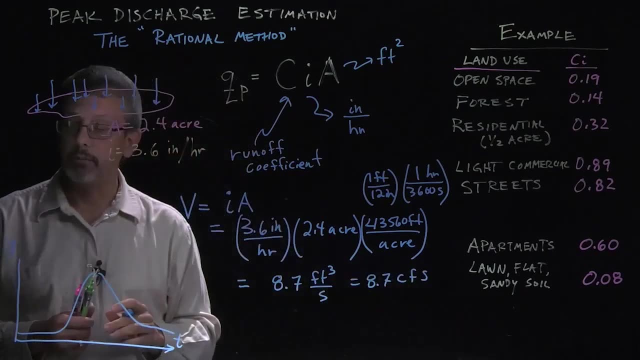 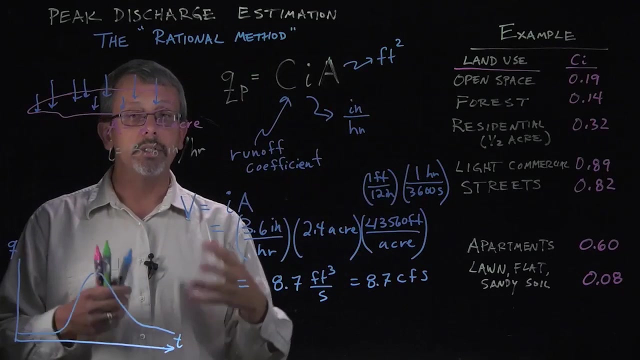 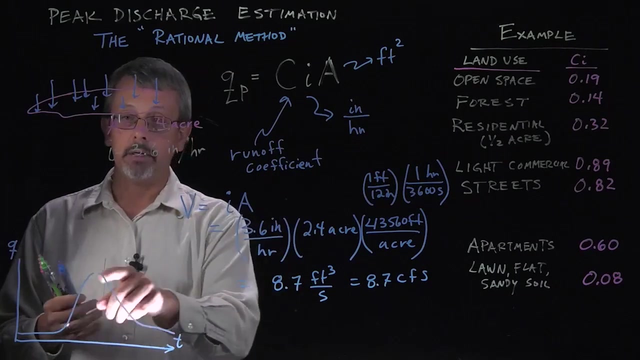 get something like eight point seven cubic feet per second or eight point seven CFS cubic feet per second. now notice this value. here is the total amount of rainfall, but only some fraction of that rainfall ends up in runoff, and ends up in runoff in the period of time necessary to contribute to this peak value. so we think about: 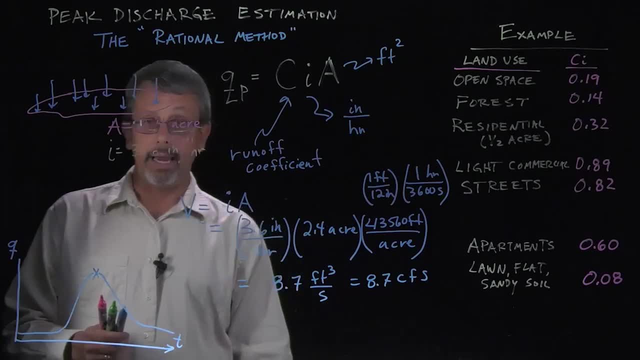 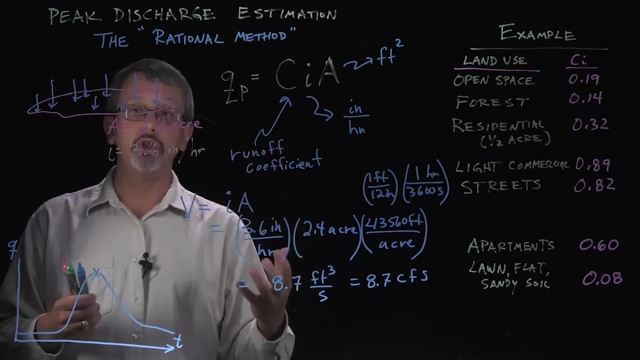 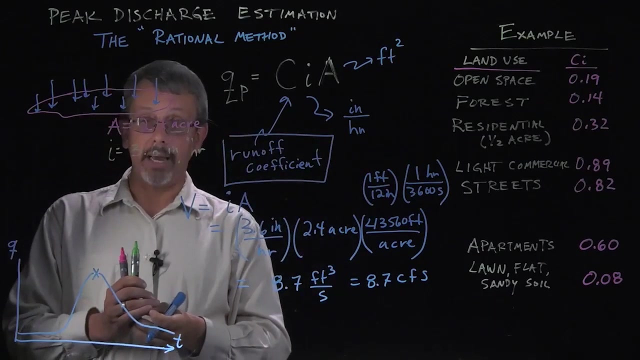 that as being some fraction. and what we do is we. this is actually an empirical relationship. what we do is we go look up on some charts. there are numerous charts that give values for this runoff coefficient and they have lots of dependencies. they depend upon things like the slope of the area, they depend upon the amount of vegetation. 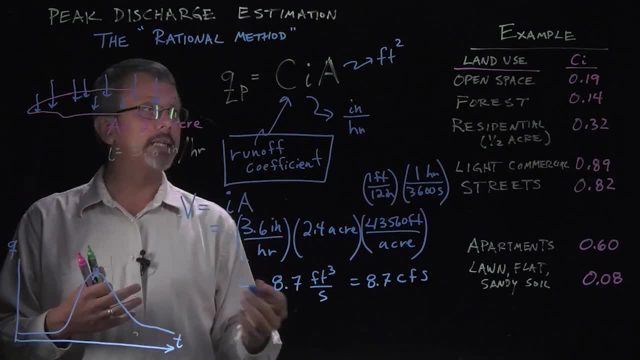 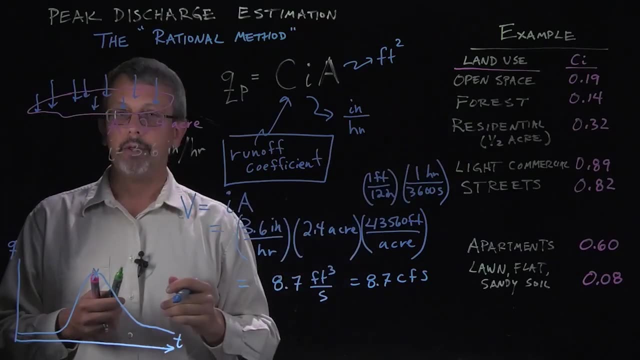 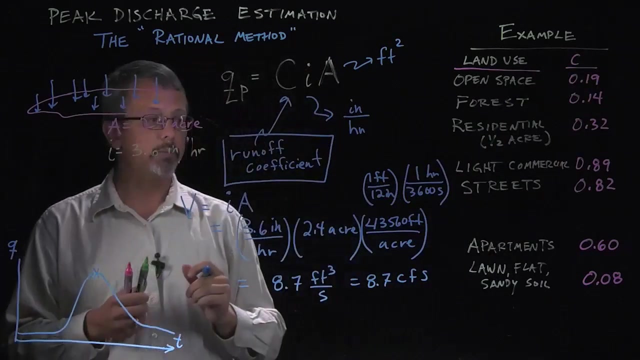 they append upon the amount of a pervious surface, for example. I have a little chart over here, okay, of a few examples of land use as compared to the coefficients, and in this particular case, I'm sorry, this C should be C sub I as, and I'll just leave it a C for the moment. okay, let's say, for example, we: 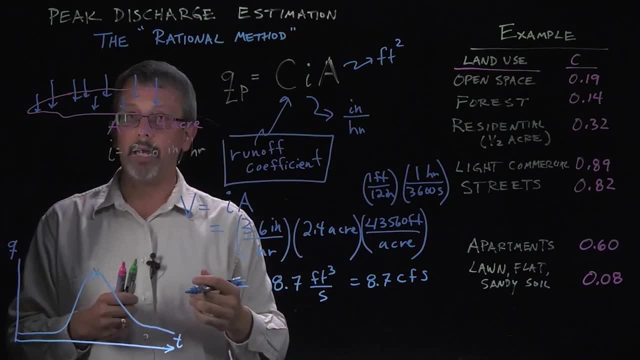 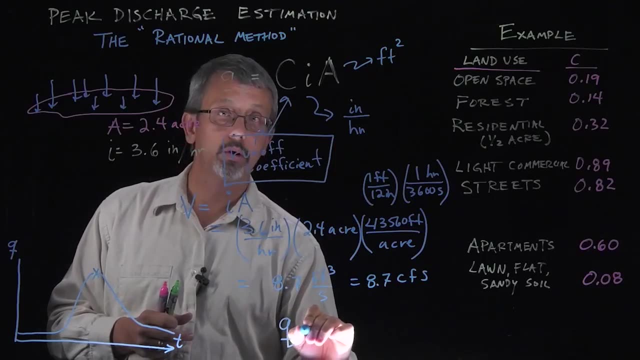 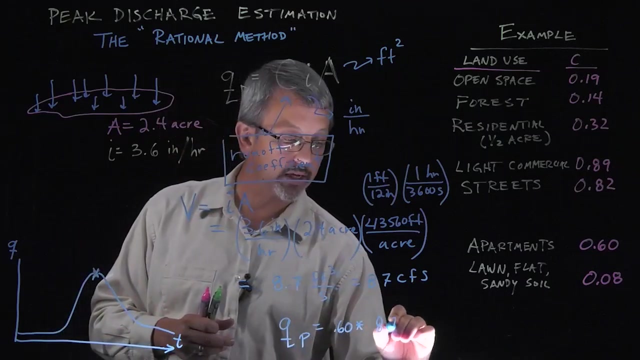 have apartments on this 2.4 acre area and we want to know what the peak overflow is going to be. well, we would simply say that our Q would be equal to point six, oh times that I a, which is the eight point seven CFS, and that would 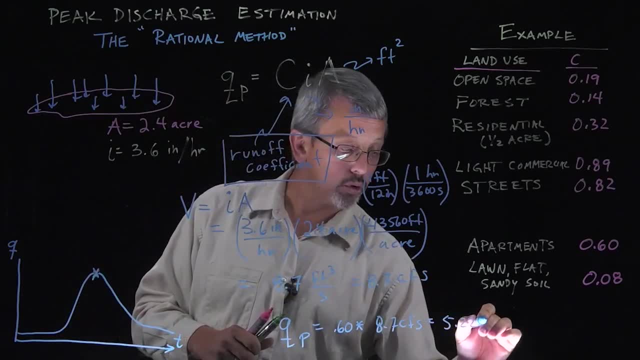 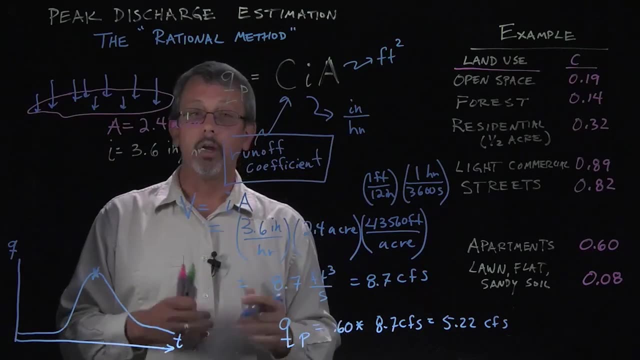 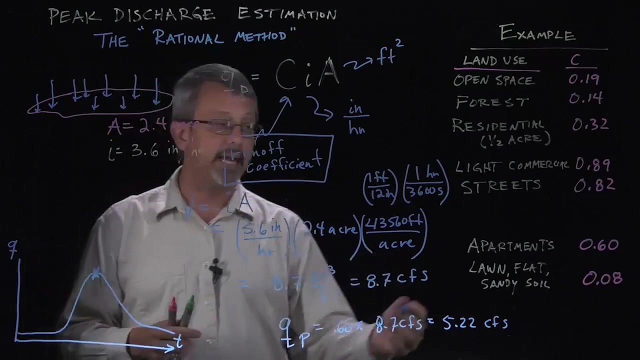 give us a value of 5.22 cubic feet per second as an estimate of this peak flow here. notice that's very different than if we have this falling on a very large 2.4 acre field. that's effectively a lawn that's maintained on flat, flat lawn maintained. 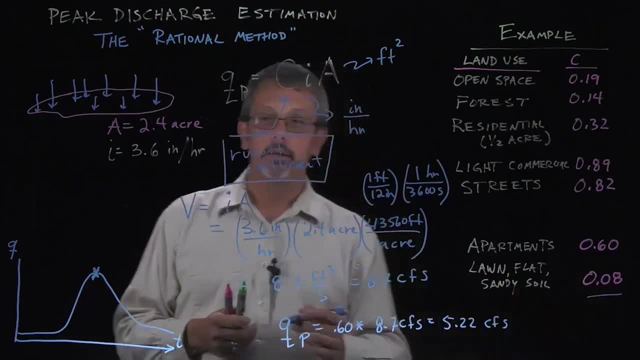 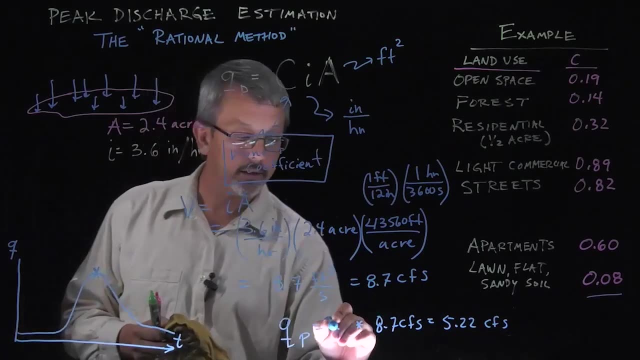 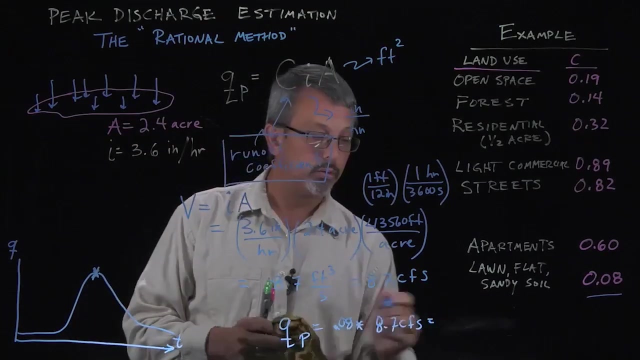 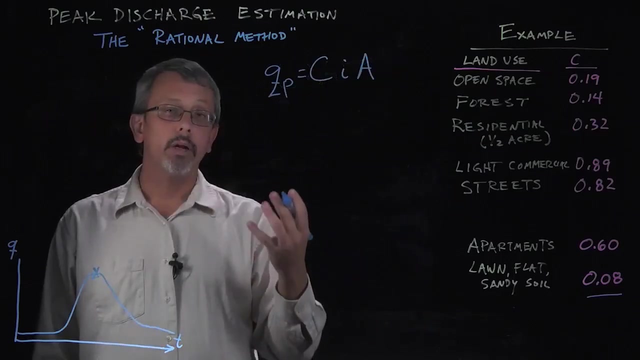 on sandy soil. in that case the coefficient has been established as being a much smaller value of point zero eight. if I plug that value in instead point zero eight, point zero eight and multiply it, I get a much smaller value of point seven O cubic feet per second. now we can apply the rational method even if we don't. 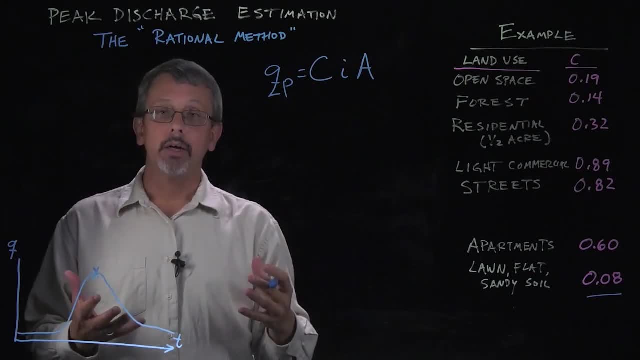 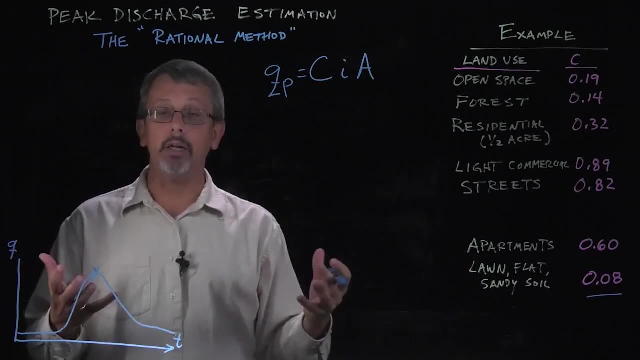 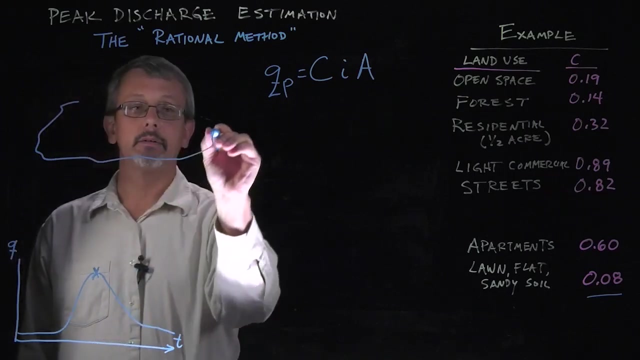 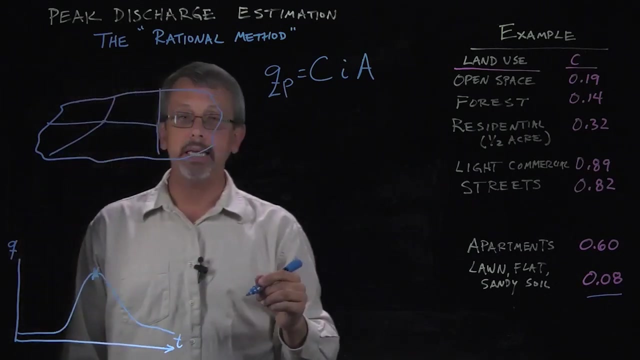 have a consistent classification of the area that we're talking about. for example, if the area you're looking at is not entirely compartments or not entirely flat lawn, we can still apply this method. by dividing up the area we're interested in into different groups or categories, for example, you might recognize that a certain piece might 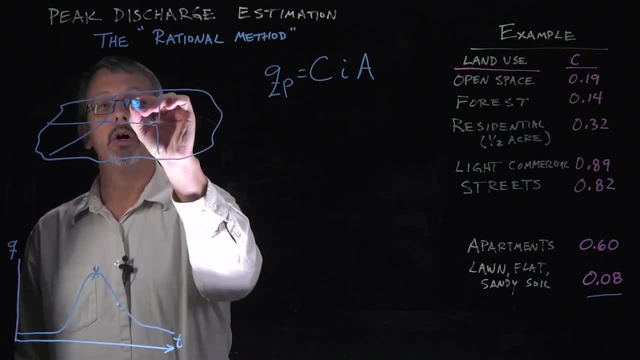 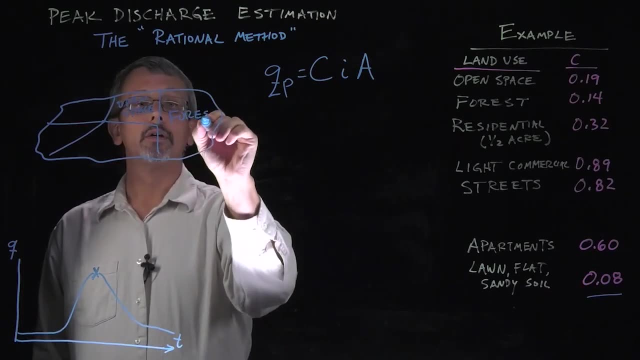 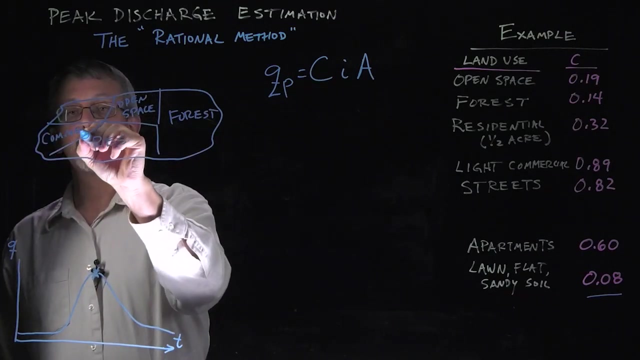 have a certain particular classification. for example, this might be open space which might about to some forest. you might have part of the area that might be residential, okay, maybe there's some commercial use over here. okay, and I'm giving some example now I've done a poor job here and that I've probably maybe 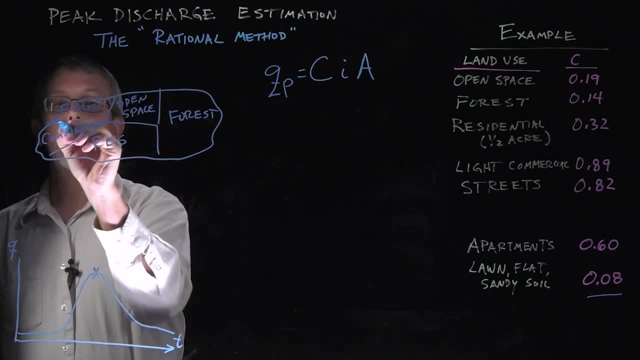 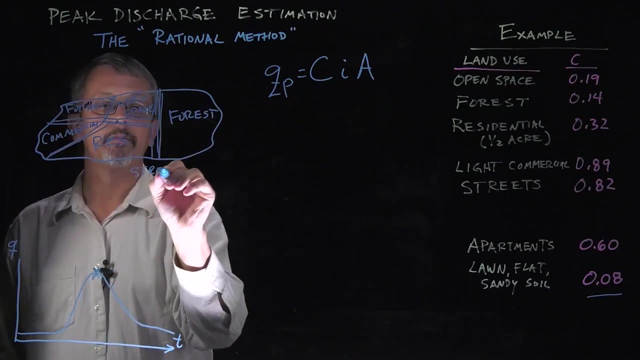 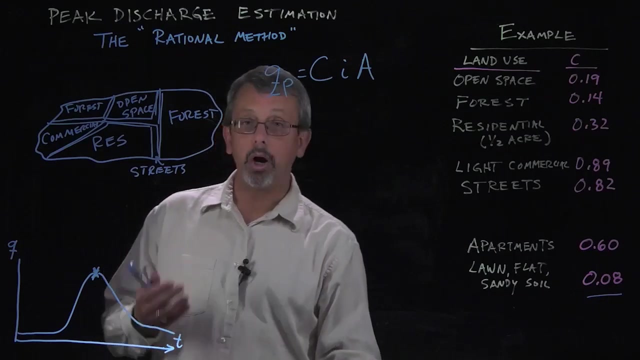 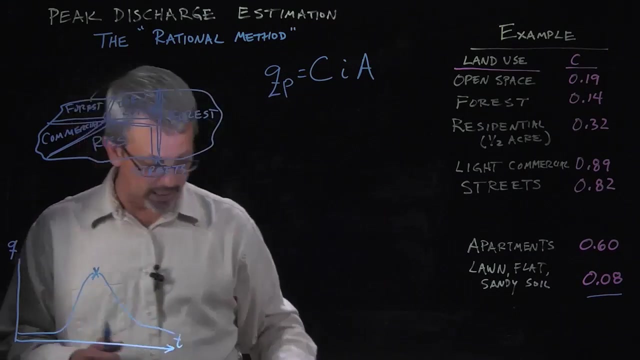 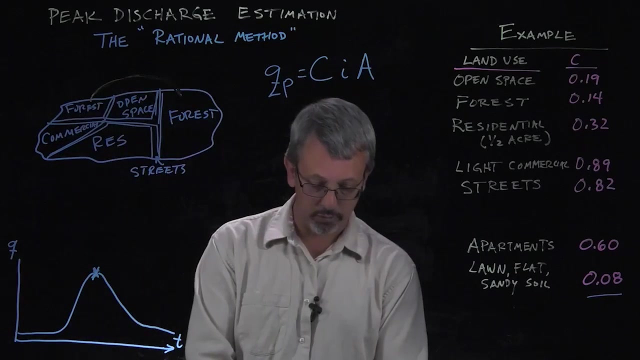 this is also forest, and then some fraction in between might represent streets, and the goal here is if you're able to associate areas, parts of the area, with each of these categories. for example, the forest might have a total amount. total area for us might have a given total area that we hope some of my markers here there might be some area. 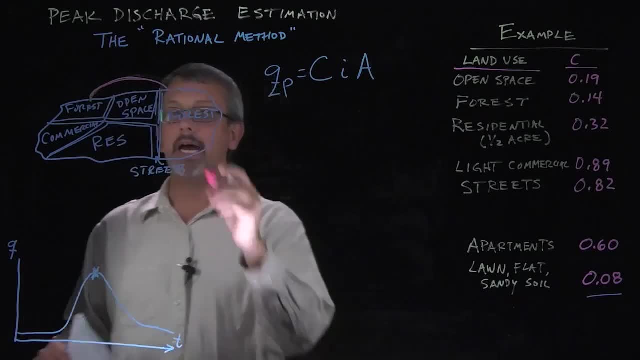 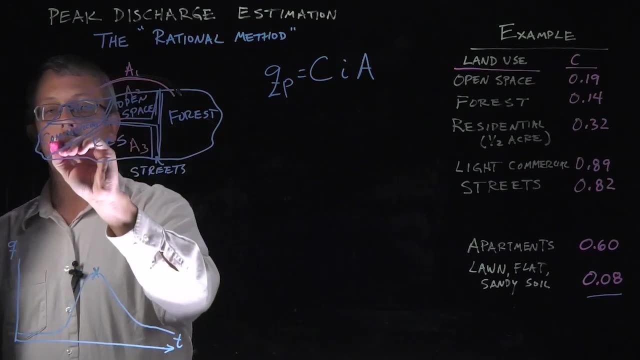 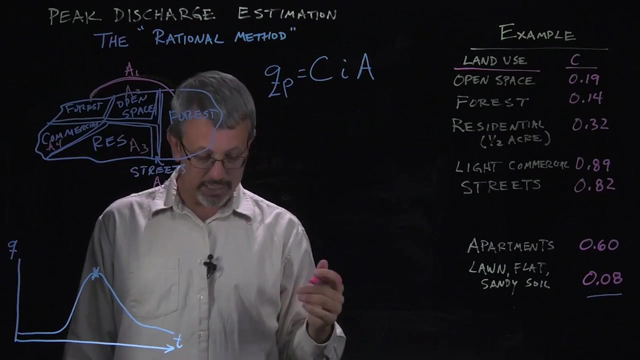 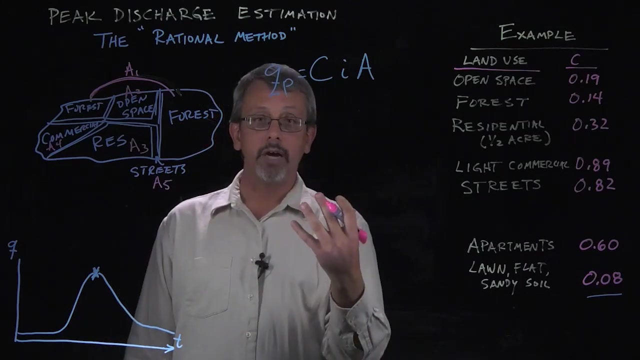 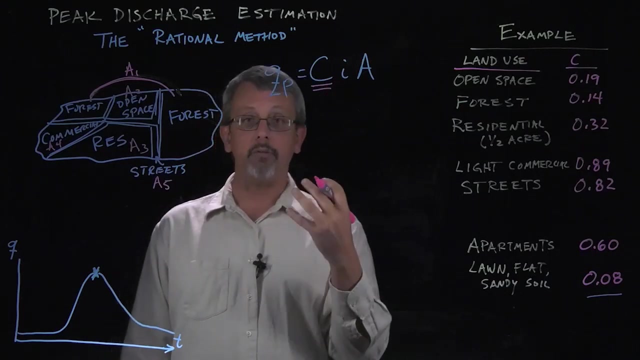 associated with the forest. maybe we can call that A1, some area associated with the open space- A2, A3, A4 and the streets: A5. If we can find the different areas associated with each of our different categories, well then what we can do is we can use area weighting to find a coefficient. 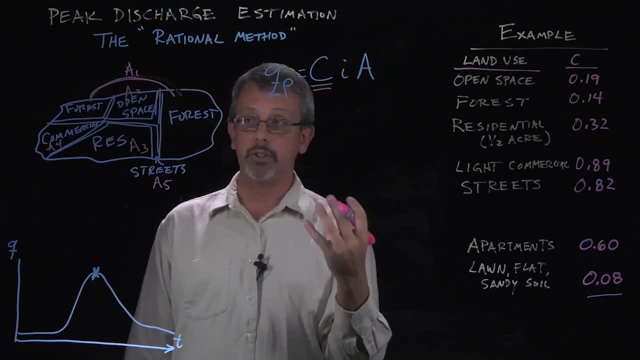 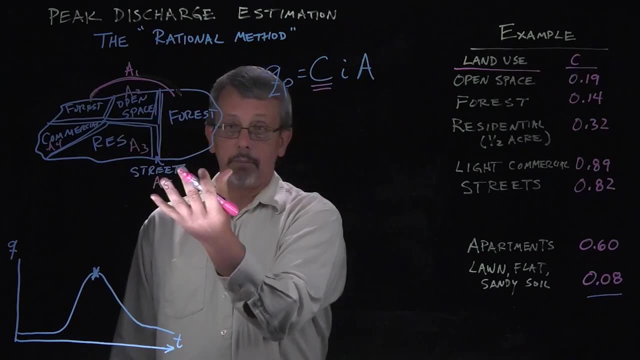 that takes into account all the different surfaces we have, But we'll need to do this by counting them based on how much area each takes up. For example, let's consider this space that I've sort of sketched here and let's assume that there are some weighting. 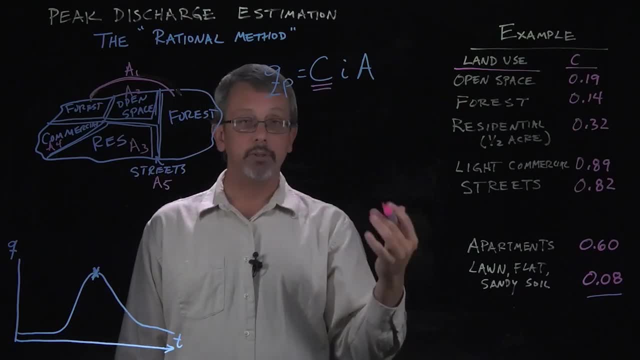 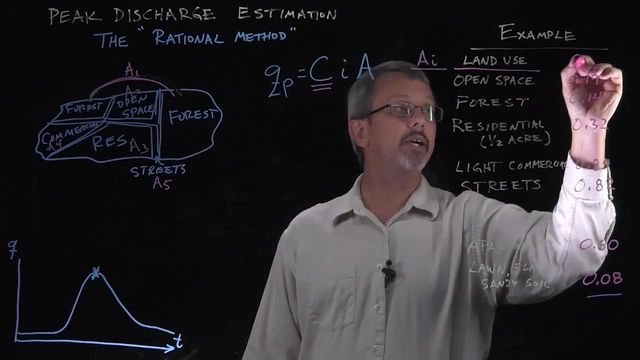 There's a different number of acres associated with each of these types of land use. For example- I'll make a list over here- AI, okay, And we have these values, CI, where I is going to be the index for each of them. 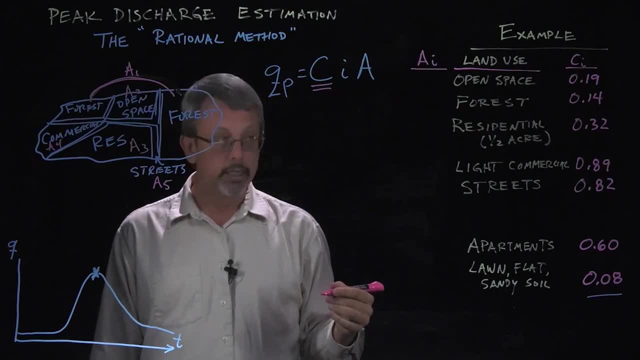 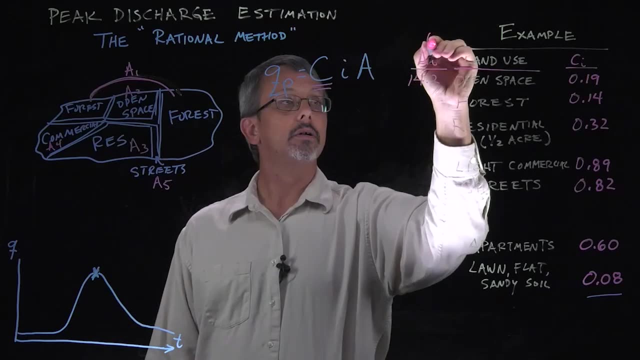 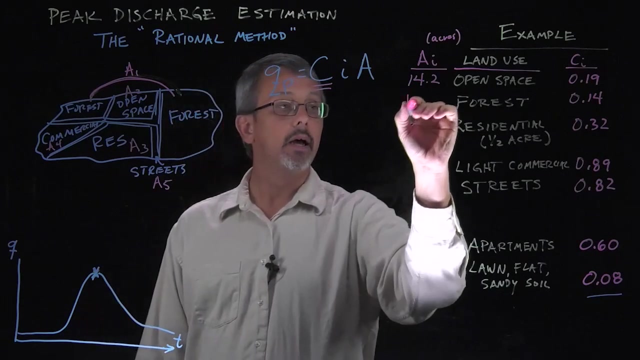 Maybe open space is one, forest is two, residential is three, and so on and so forth. So we have the different coefficients and let's assume that we measure the acreage Associated with each of these. For example, 14.2 acres of open space, 11.6 acres of forest, 8.9 acres of residential. 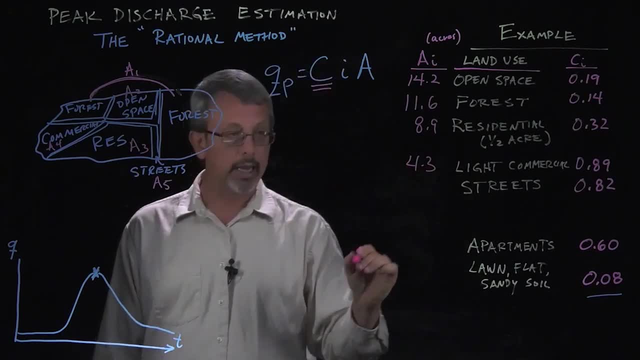 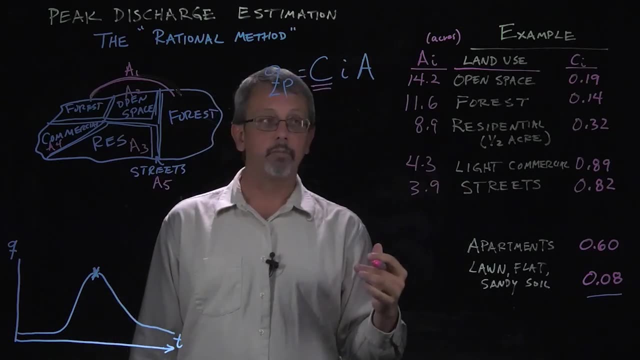 4.3 acres of light commercial and 3.9 acres of street, So there are different values associated with each of these different areas. Well, what we're going to do to define the C that we're going to use here is: we're going to use the C that we're going to use here. 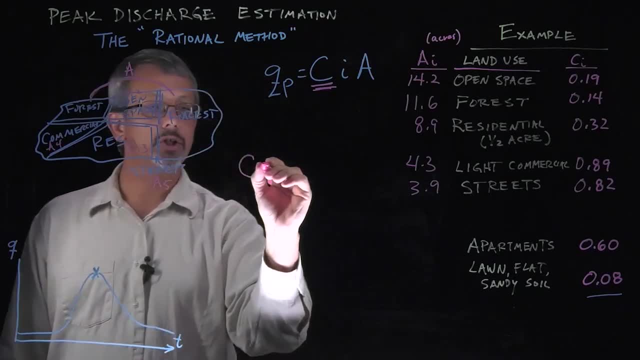 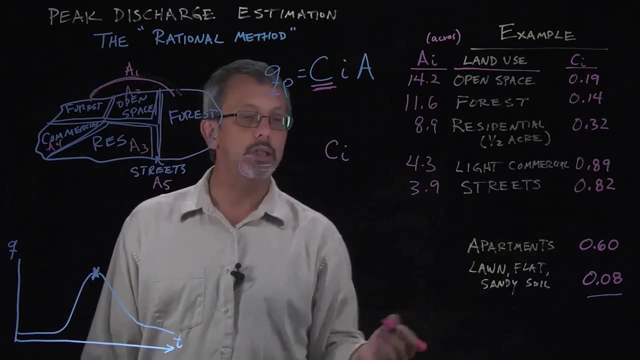 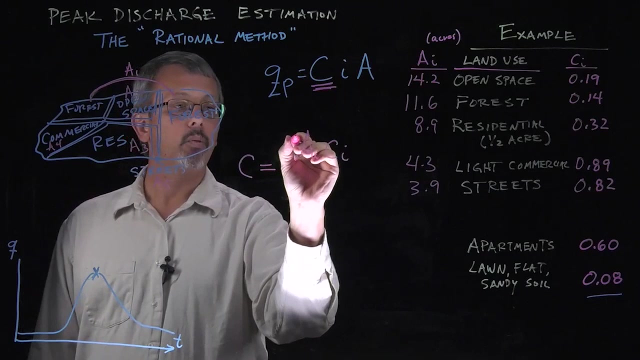 This coefficient is. we're going to create a weighted average. We're going to take each coefficient I, the list of coefficients that corresponds with each type, we're going to multiply it by the area that's associated with it And then we're going to sum all of those values. 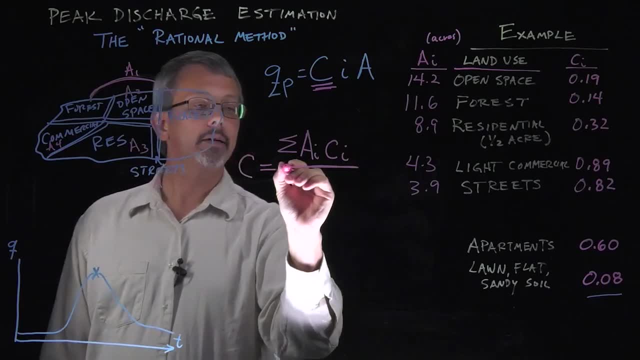 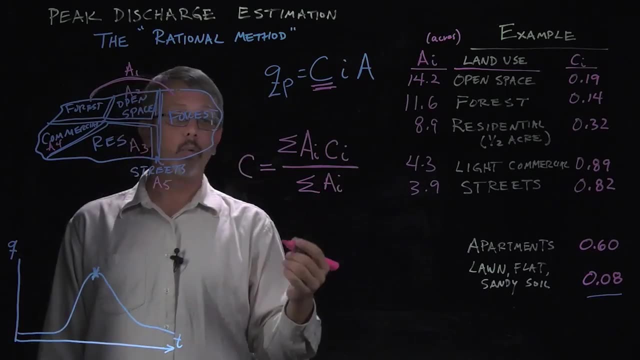 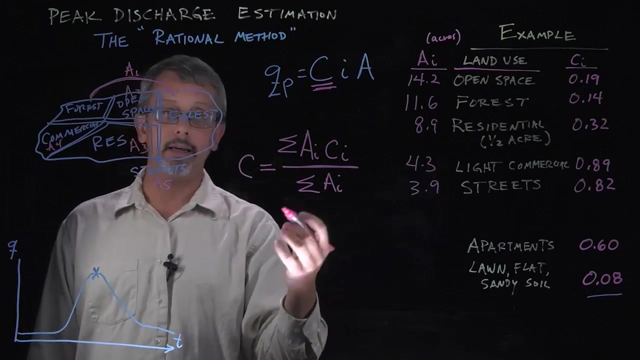 After we've done that, we're going to normalize again by taking the sum of all the areas dividing out by the total area. In other words, you can think of each of these pieces as being a fraction that it contributes Each. the forest contributes A1 over the total, A as a fraction of the coefficient. 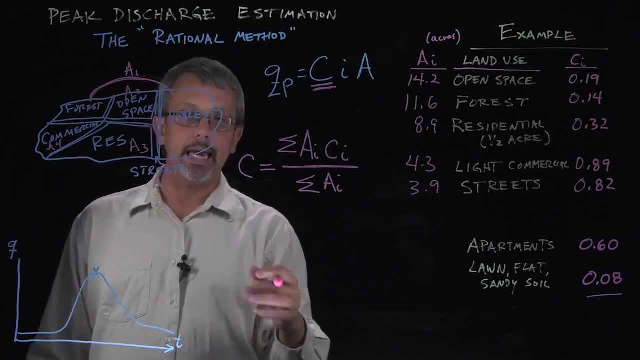 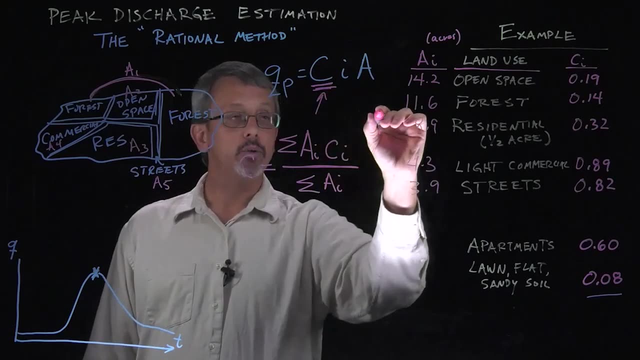 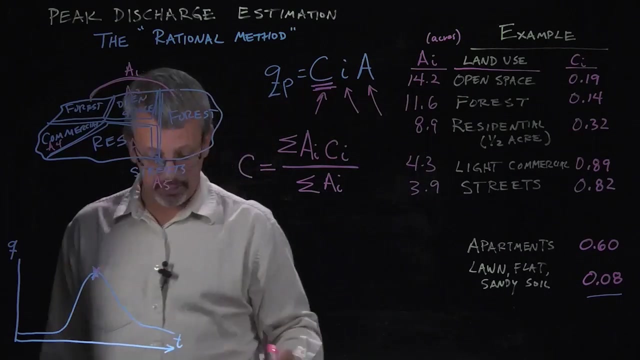 If I do this calculation here, then I will get a weighted average coefficient. That coefficient is the one that we can then plug in here and use the overall area and the overall rainfall intensity to estimate the total area. We're going to setup all of these by thing outbreak units. 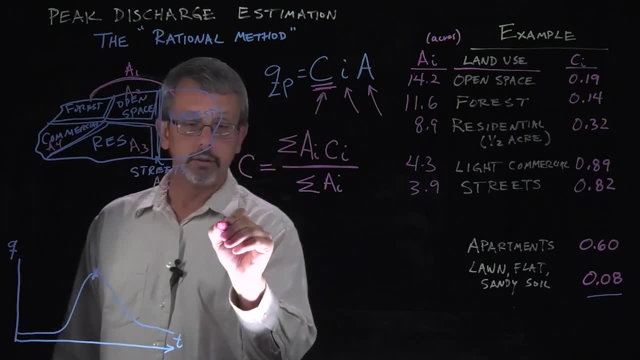 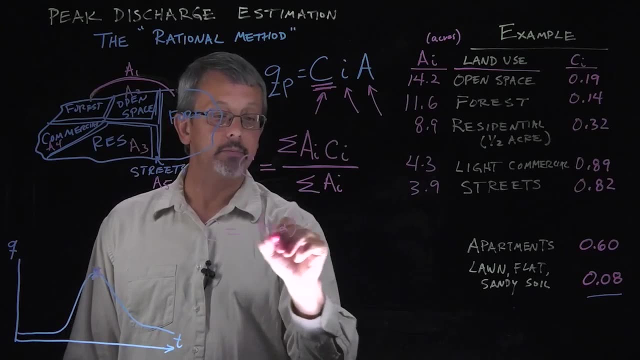 and then we're going to add these by thing- accident risk- and then then we would take your rate of additional targets per unit. Now the unit for hospitalization is the unit impact, the unit patient health rate, the unit vehicle fuel capacity.